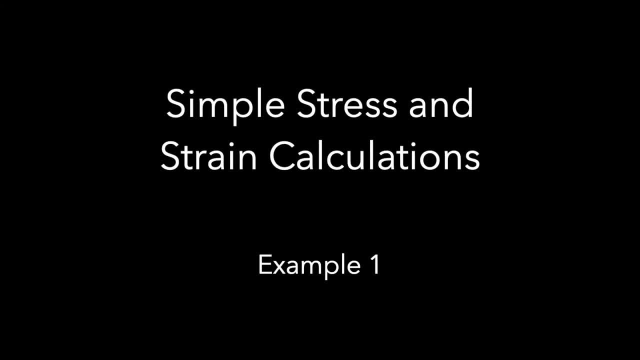 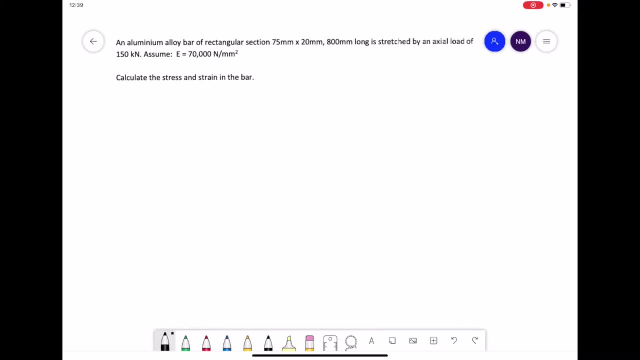 In this problem. we have an aluminium alloy bar of rectangular cross section, 75 by 20 mils, 800 millimeters long and is stretched by an axial load of 150 kilonewtons. Young's modulus is 70 000 newtons per millimeter squared. Here we have to calculate the stress and the strain in the bar. 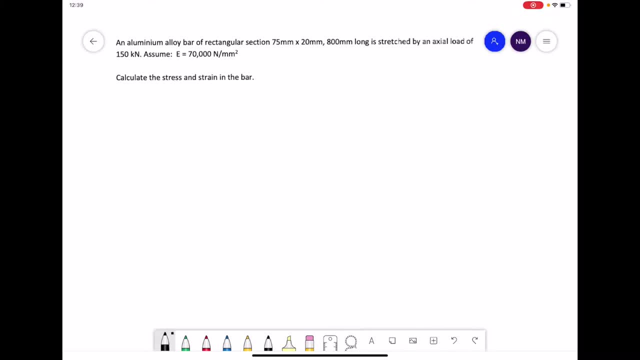 The first thing we're going to do is to draw a little diagram to represent the problem. It doesn't have to be drawn to scale. This is our bar. The overall length is 800 millimeters and load is applied stretching the bar In section. the bar is 75 by 20 millimeters. 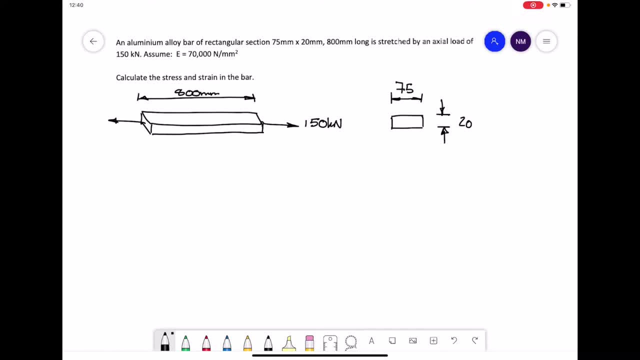 First thing we can do is to calculate the stress on the bar and the equation for stress is: stress is going to be force over area, or stress sigma is f over. a force we have is 150 kilonewtons, so we'll convert that to newtons, so it's 150: 000. divide that by the cross-sectional area and that would be the 75. 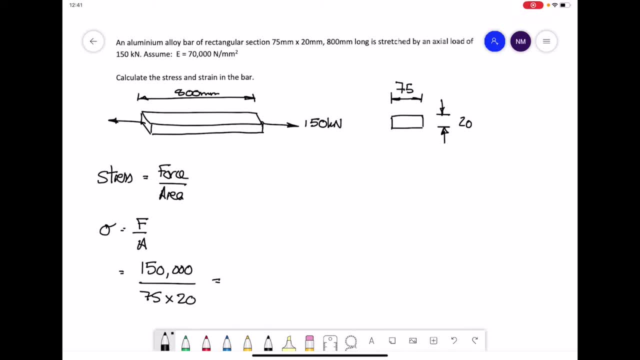 by 20, and that would give you a stress of 100 newtons per millimeter squared. Next, we have to calculate the strain, and the equation we normally use for strain is: strain is the change in length over our original length. However, we don't have the change in length. we do have the original length, but with only knowing one.